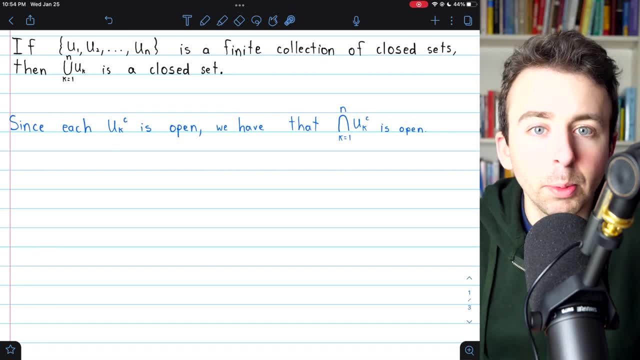 complement which is open By definition. the complement of a closed set has to be an open set. Then we could imagine taking the intersection of this finite collection of open sets. Take the complement of every one of these closed sets and we'll have a finite collection of open sets And we 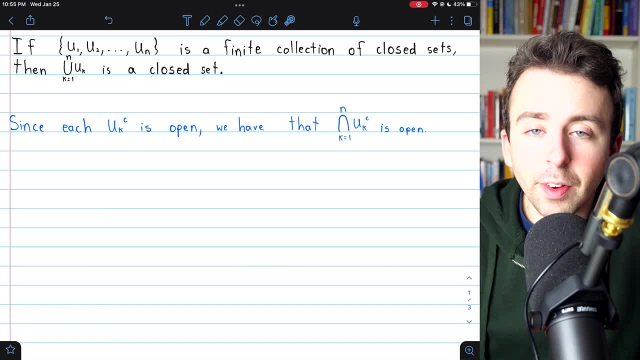 could take their intersection, And we've already proven that a finite intersection of open sets is also open. So this finite intersection of open sets, of course, is open. Now, if we take the complement of this finite intersection, we will get a closed set because 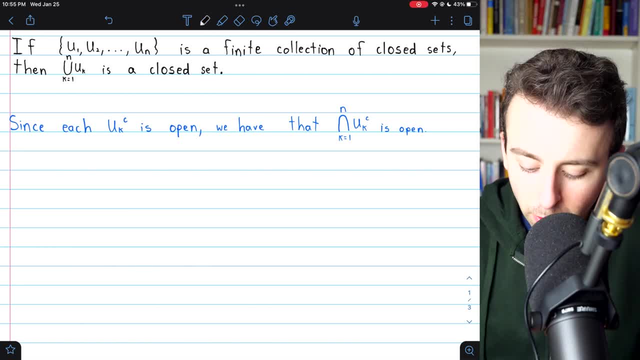 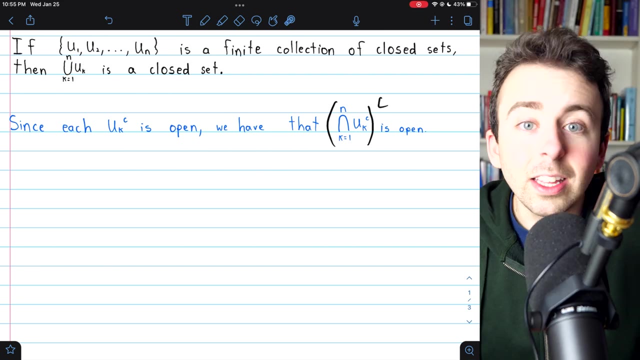 by definition, the complement of an open set is closed. So we're going to take the of this open set to get a closed set. but as it turns out by De Morgan's laws, the complement of this finite intersection is exactly the finite union that we're trying to prove our result about. 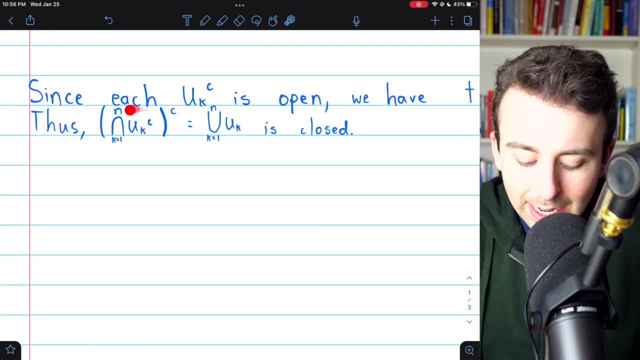 and that is because, when we take the complement of this finite intersection, each intersection becomes a union and each complement of the closed sets right, each UK complement becomes the original closed sets UK and again, since this is the complement of an open set, it has to be closed. 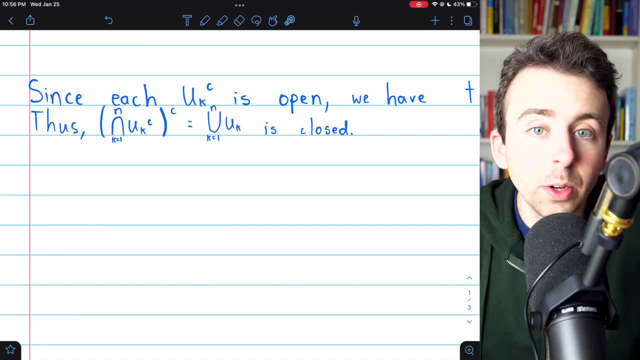 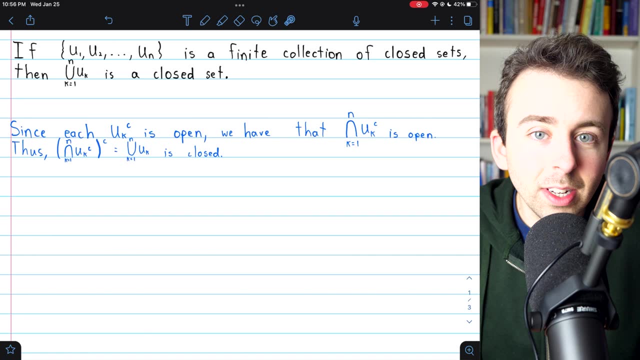 so we've proven that this finite union of our closed sets is closed Once more. the fact that the complement of this open set is closed is just by definition, but the fact that the complement of this open set equals this union of closed sets is a result of De Morgan's law and the proof. 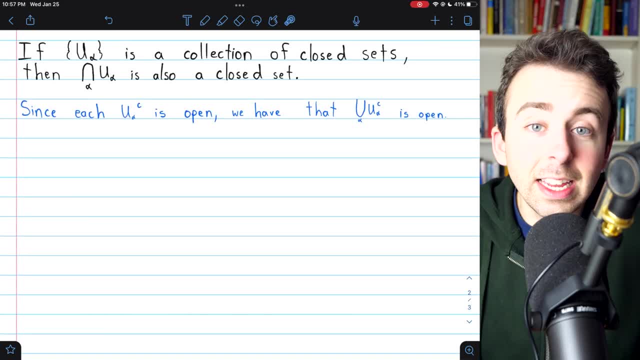 for an arbitrary intersection of closed sets is very similar. We could take the complement of any one of these closed sets and certainly say U-alpha complement. it would have to be open because the complement of a closed set is open. but then we could consider the arbitrary union. 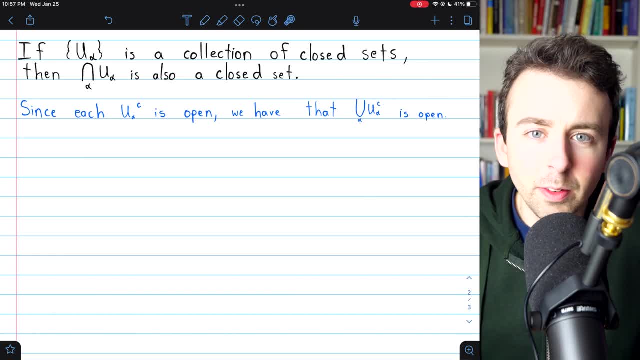 of all of these open sets, the union of every U-alpha complement. By a previous proof, we know that the union of every U-alpha complement has to be open, because if we take the complement of this arbitrary union, we will by definition get a closed set, but again by De Morgan's law.